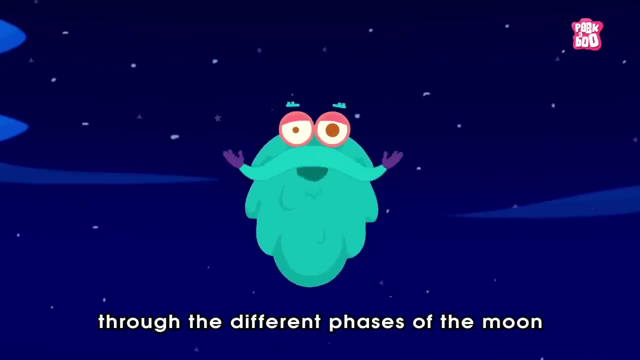 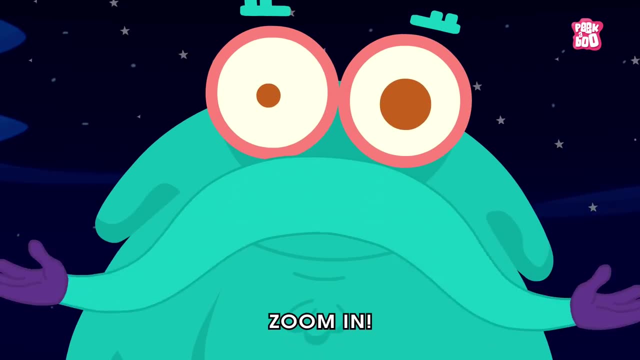 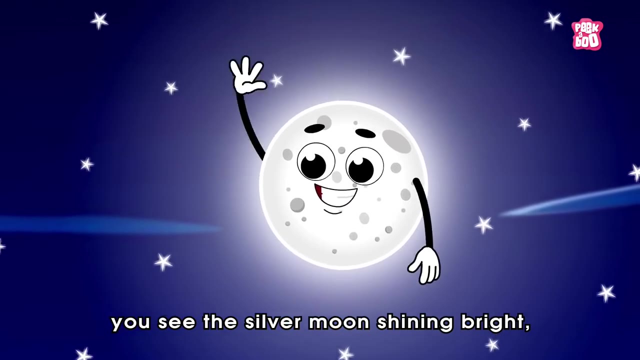 So in today's episode, let me take you through the different phases of the Moon and shed some light on the reasons behind it. Zoom in, Hey friends. every time you look up in the sky at night, you see the Silver Moon shining bright, illuminating the Earth from its light. 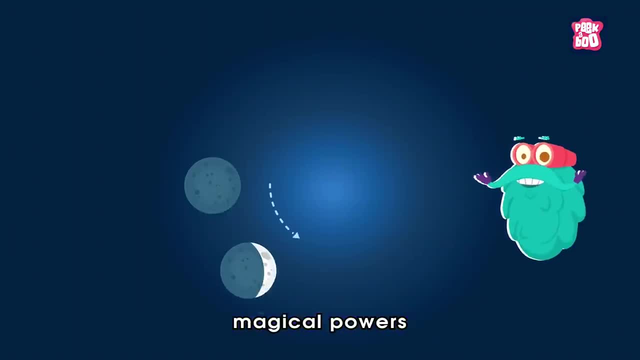 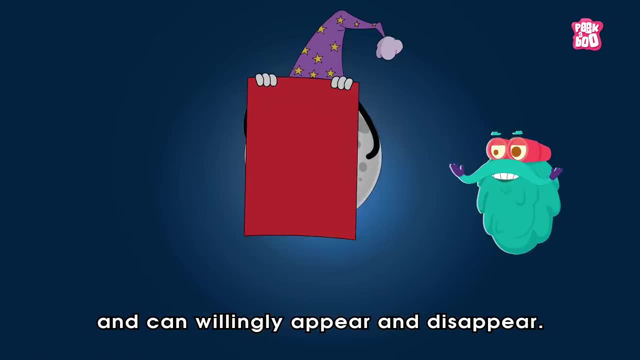 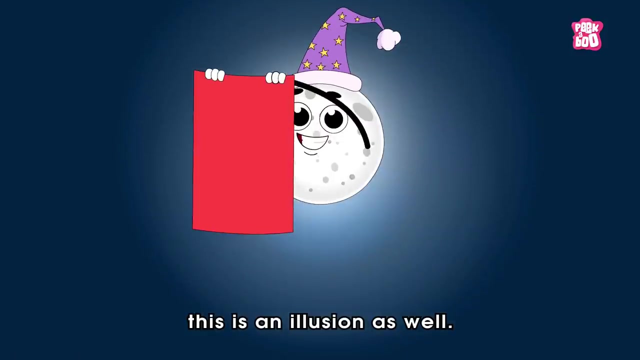 Not only that, but the Moon also seems to have magical powers to change its shape and can willingly appear and disappear. But the matter of fact is, like any magic trick, this is an illusion as well. Yes, my dear friends, you will be surprised to know. 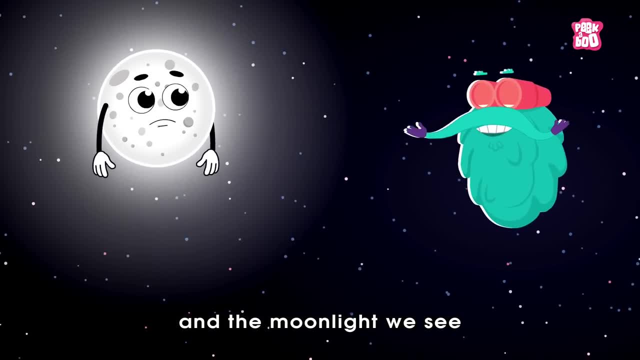 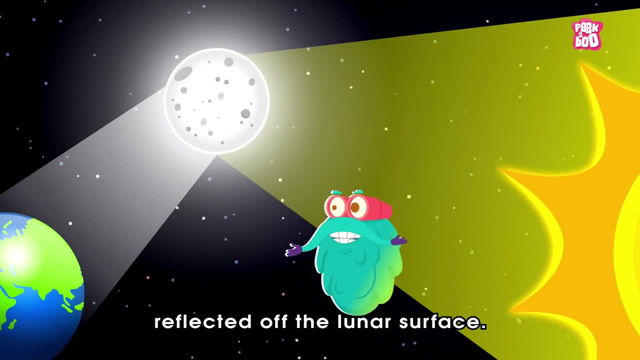 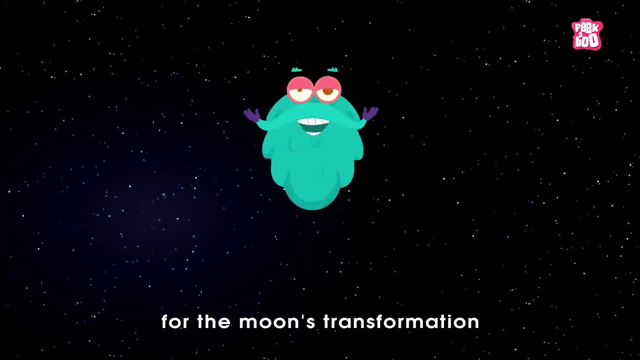 that the Moon doesn't emit light itself and the Moonlight we see is actually the Sun's light reflected off the Luna's surface. Yes, this Sunlight is also responsible for the Moon's transformation from the New Moon to the Full Moon and back again. 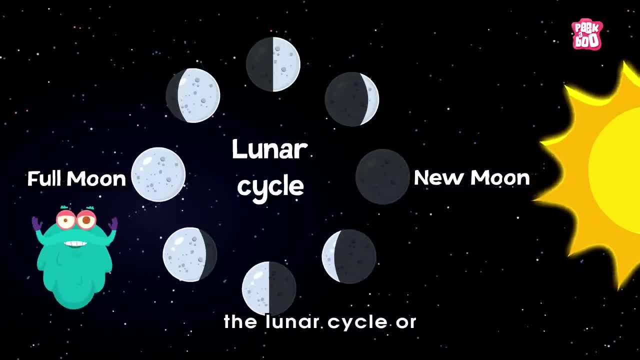 Under the process, we call the Luna Cycle or the Phases of the Moon. Under the process, we call the Luna Cycle, or the Phases of the Moon. Under the process, we call the Luna Cycle or the Phases of the Moon. 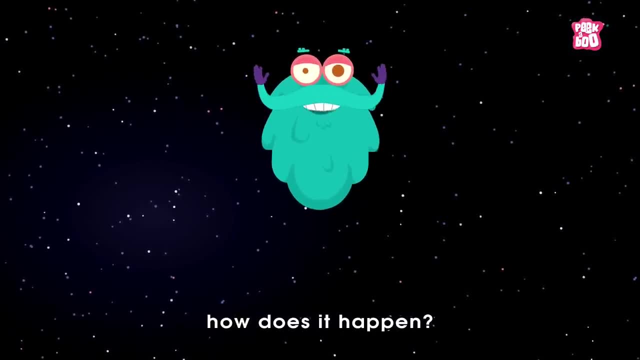 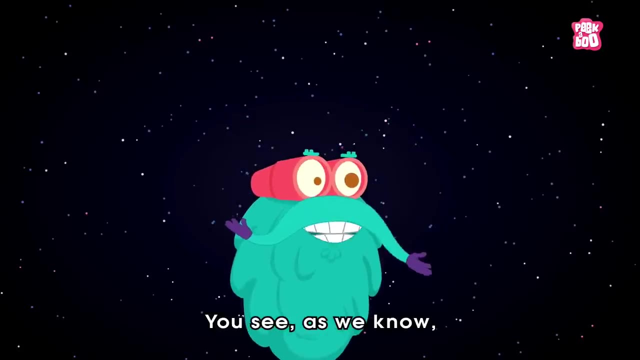 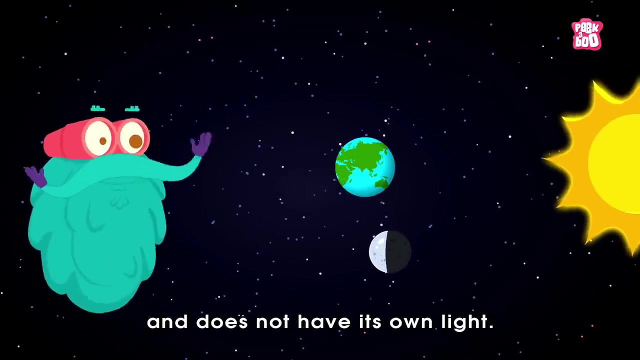 But the vital question is: how does it happen? So let us have a good look at it. You see, as we know, the Moon revolves around the Earth at a fixed orbit and does not have its own light. So when the Moon is exactly in the middle of the Earth and the Sun, 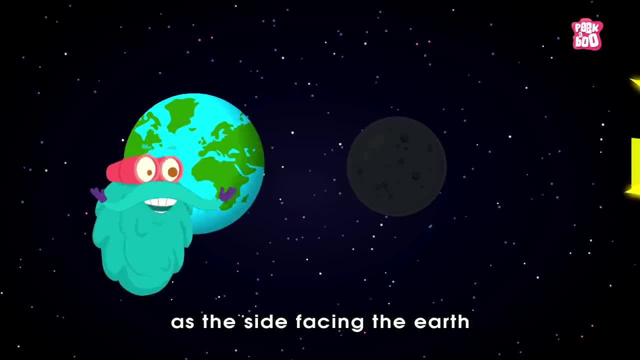 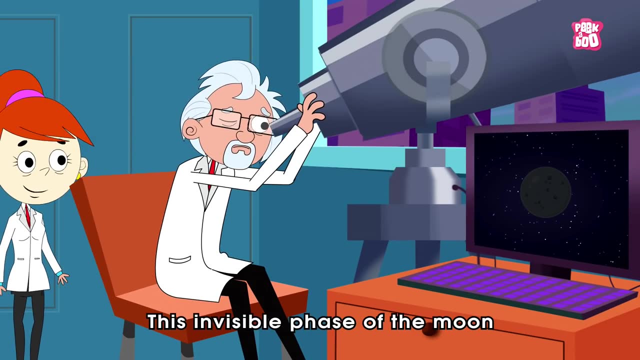 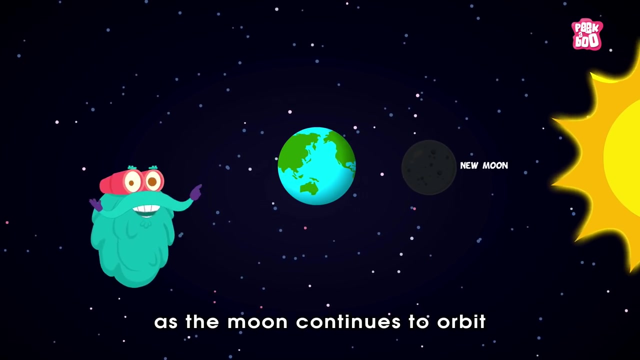 it becomes nearly invisible in the night sky as the side facing the Earth does not get the Sunlight. This invisible Phase of the Moon is called the New Moon, But as the Moon continues to orbit and moves a little ahead in the waxing Phase, 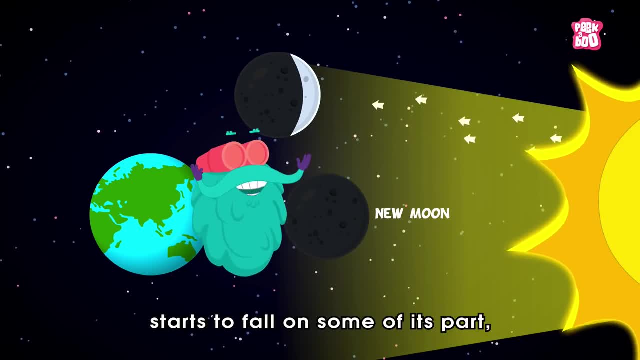 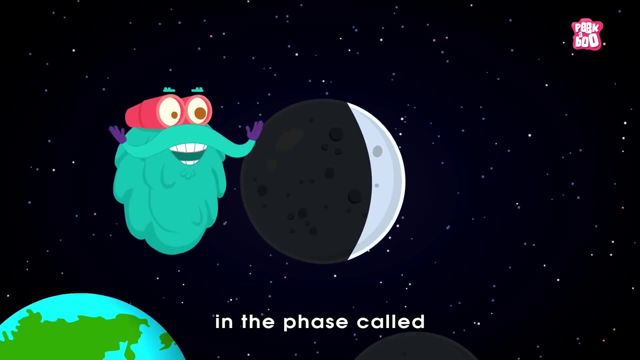 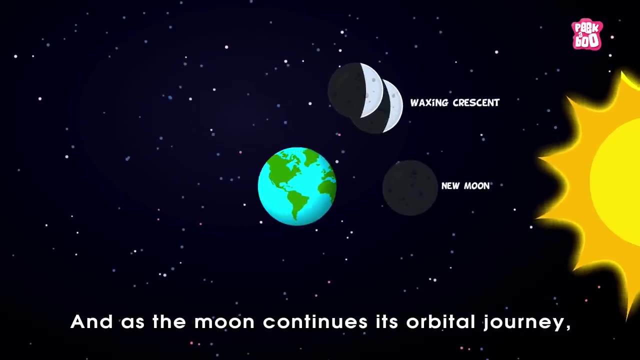 after two or three days, some light from the Sun starts to fall on some of its part, which makes the Moon appear in a crescent shape in the Phase called the Waxing Crescent. And as the Moon continues its orbital journey, the Sun's reflection keeps on increasing on the Moon's surface. 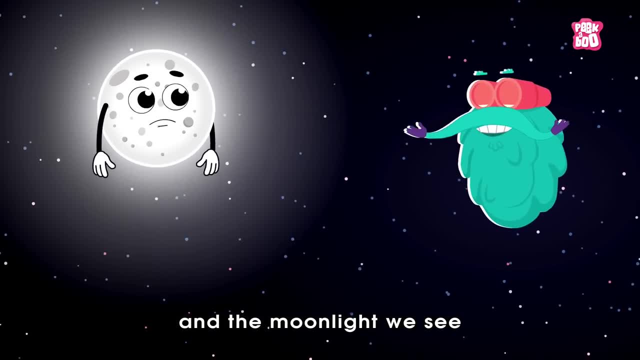 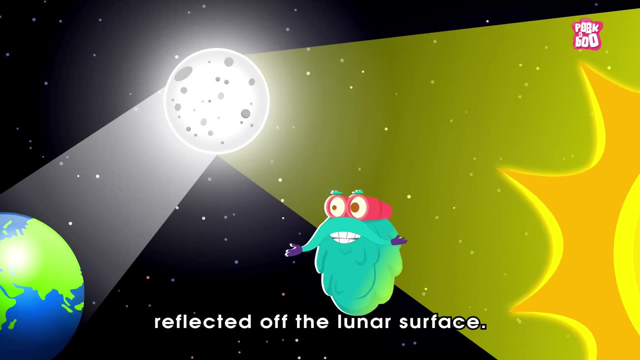 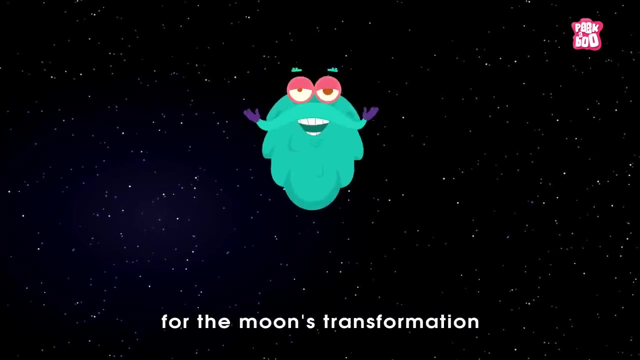 that the Moon doesn't emit light itself and the Moonlight we see is actually the Sun's light reflected off the Luna's surface. Yes, this Sunlight is also responsible for the Moon's transformation from the New Moon to the Full Moon and back again. 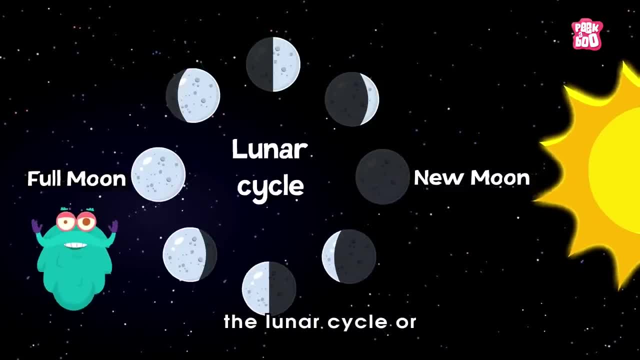 Under the process, we call the Luna Cycle or the Phases of the Moon. Under the process, we call the Luna Cycle, or the Phases of the Moon. Under the process, we call the Luna Cycle or the Phases of the Moon. 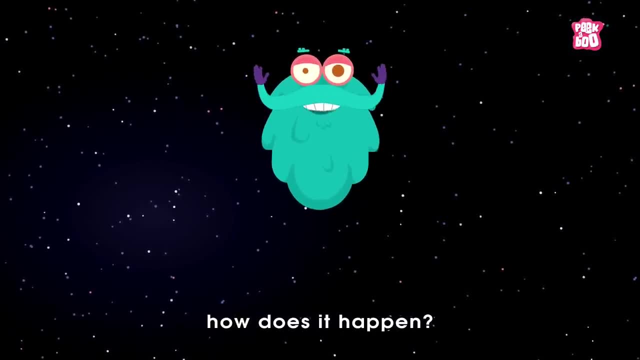 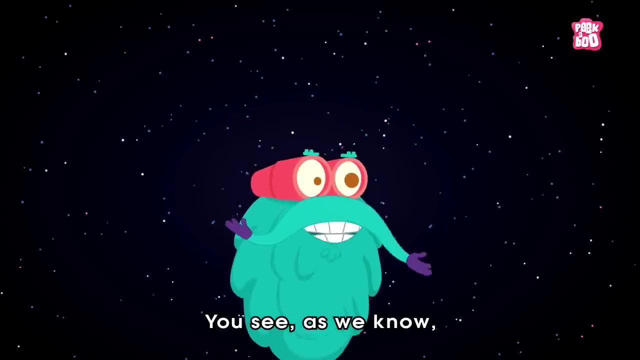 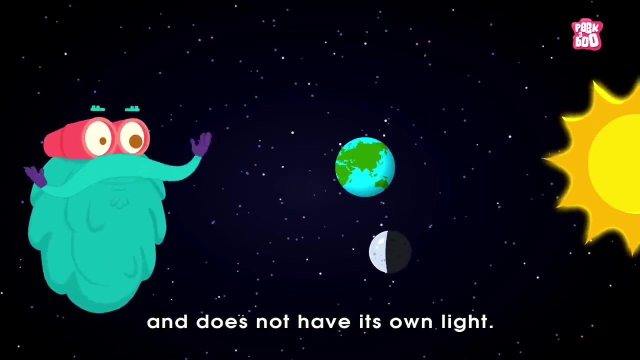 But the vital question is: how does it happen? So let us have a good look at it. You see, as we know, the Moon revolves around the Earth at a fixed orbit and does not have its own light. So when the Moon is exactly in the middle of the Earth and the Sun, 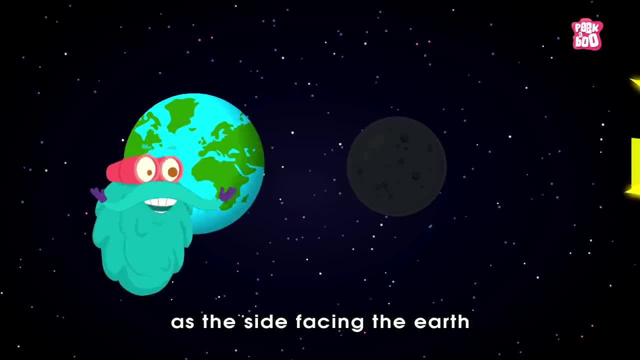 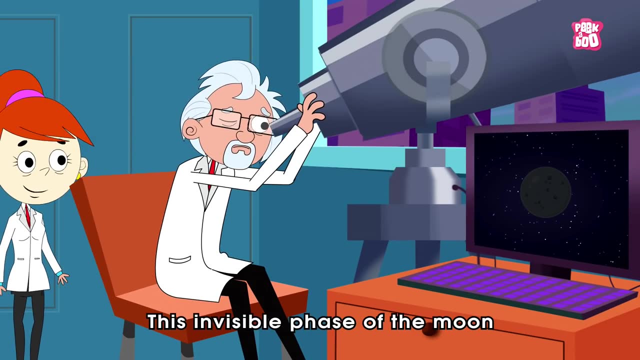 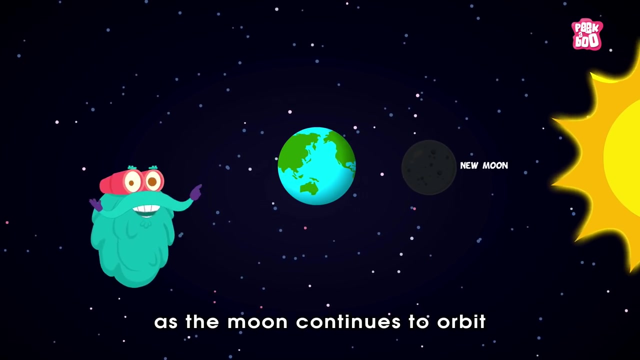 it becomes nearly invisible in the night sky as the side facing the Earth does not get the Sunlight. This invisible Phase of the Moon is called the New Moon, But as the Moon continues to orbit and moves a little ahead in the waxing Phase, 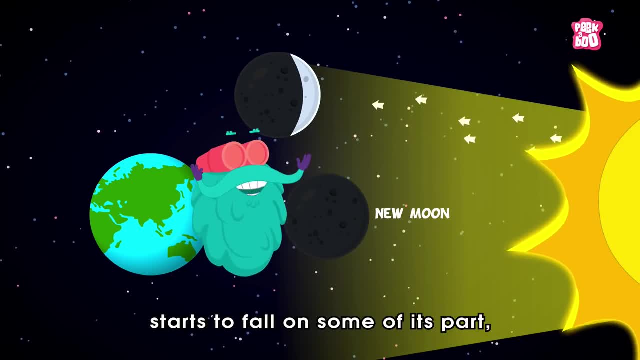 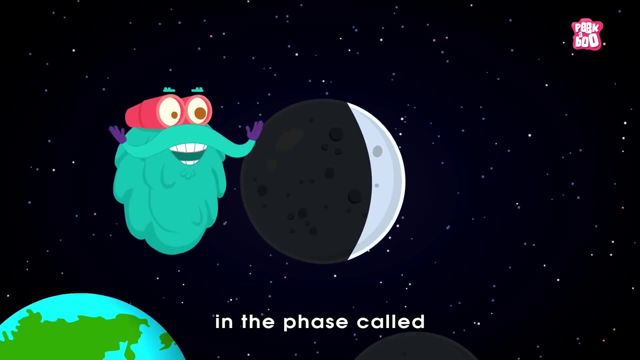 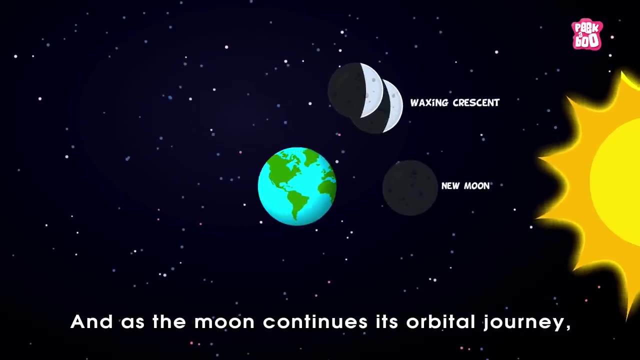 after two or three days, some light from the Sun starts to fall on some of its part, which makes the Moon appear in a crescent shape in the Phase called the Waxing Crescent. And as the Moon continues its orbital journey, the Sun's reflection keeps on increasing on the Moon's surface. 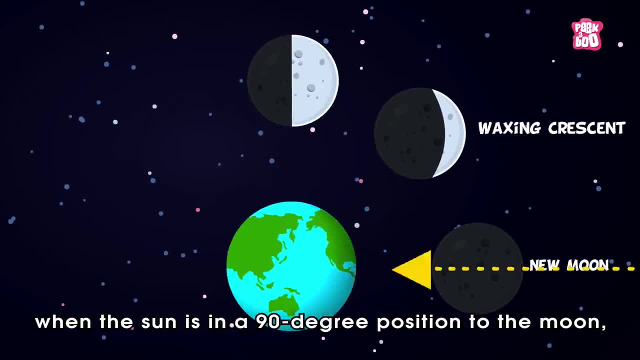 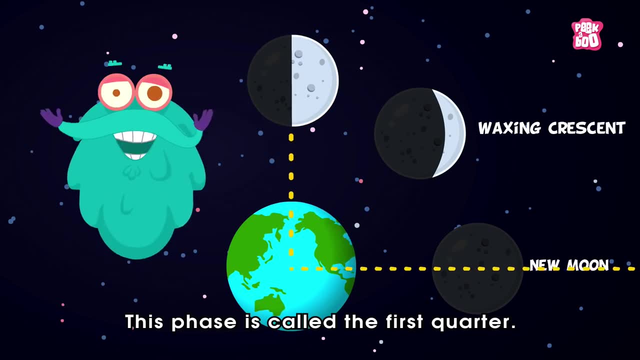 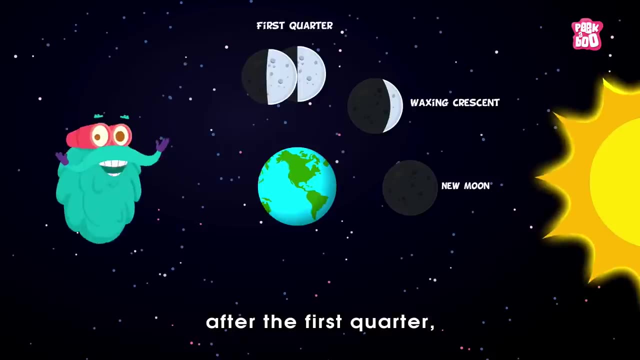 And in about a week, when the Sun is in a 90 degree position to the Moon, we could see its half-lit portion. This Phase is called the First Quarter. Next in about two or three days after the First Quarter. 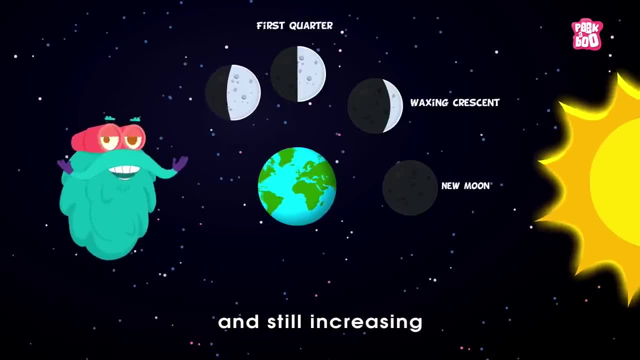 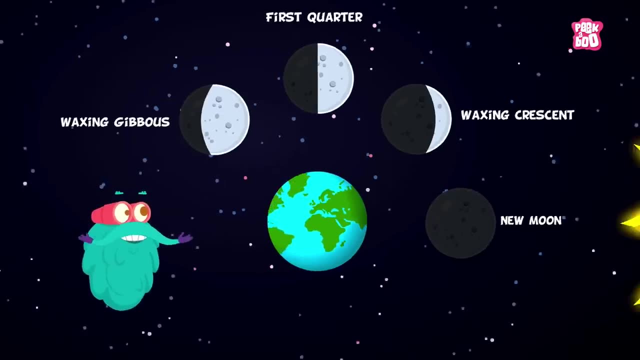 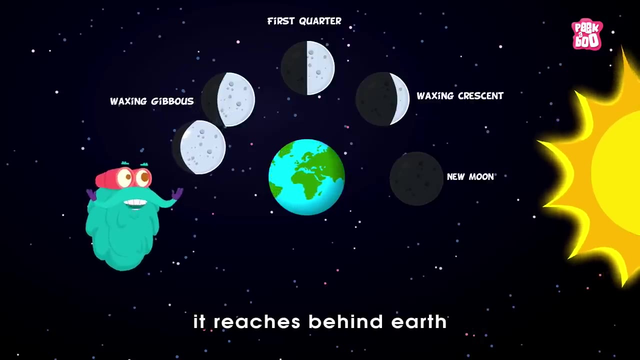 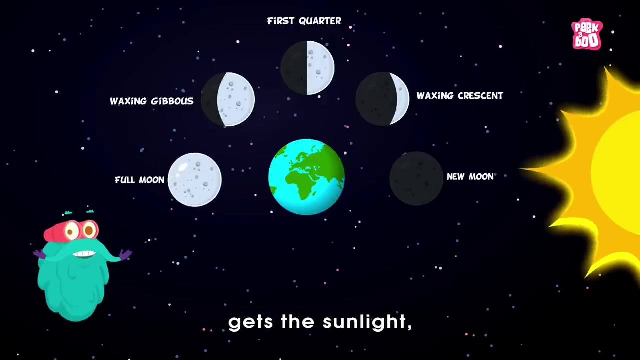 the Moon is more than half-full and still increasing its illuminated surface in the Phase we called Waxing Gibbous, And in about two weeks after the New Moon or the Invisible Moon, it reaches behind Earth with respect to the Sun, and the full side of the Moon facing the Earth gets the Sunlight. 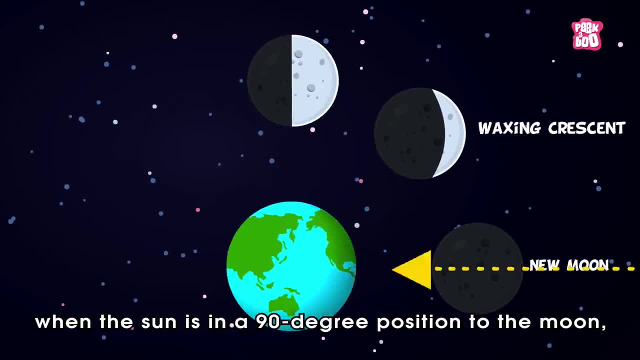 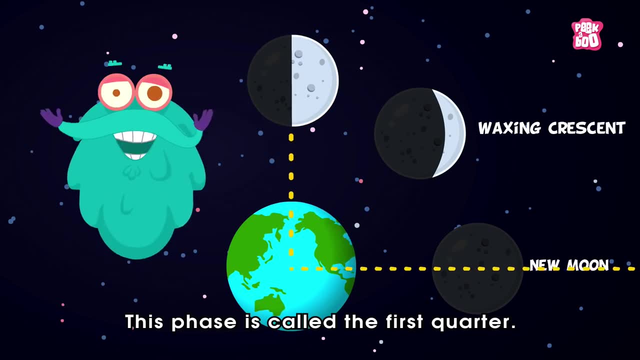 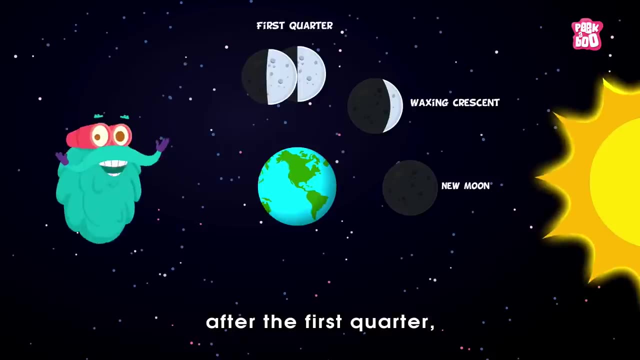 And in about a week, when the Sun is in a 90 degree position to the Moon, we could see its half-lit portion. This Phase is called the First Quarter. Next in about two or three days after the First Quarter. 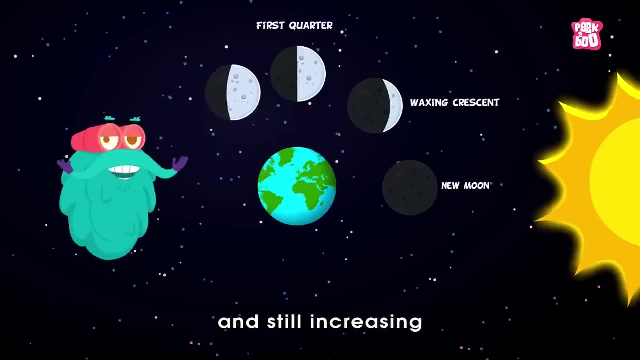 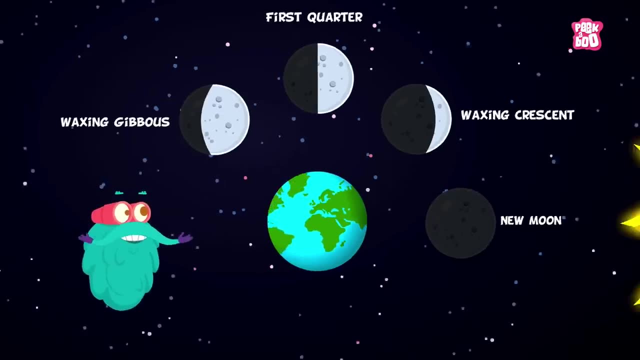 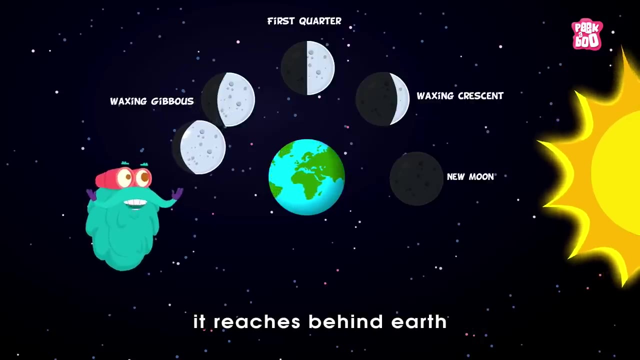 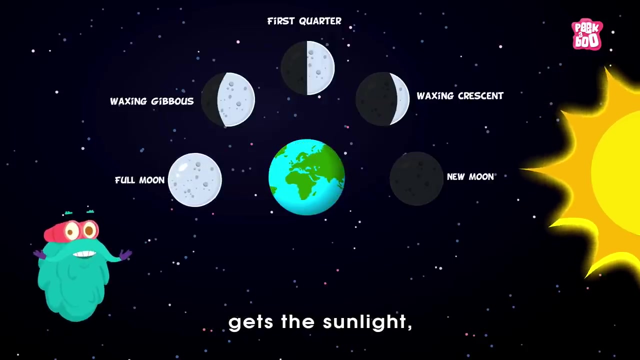 the Moon is more than half full and still increasing its illuminated surface in the Phase we called Waxing Gibbous, And in about two weeks after the New Moon, or the Invisible Moon, it reaches behind Earth with respect to the Sun, and the full side of the Moon facing the Earth gets the Sunlight. 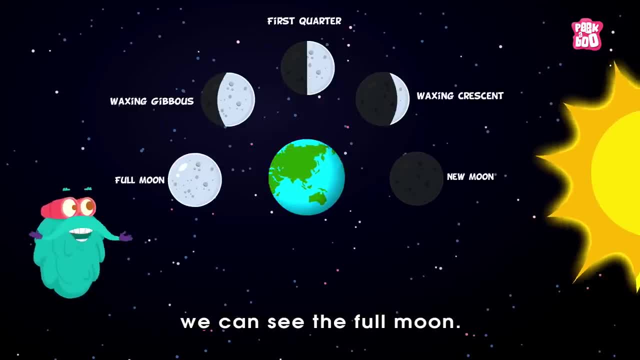 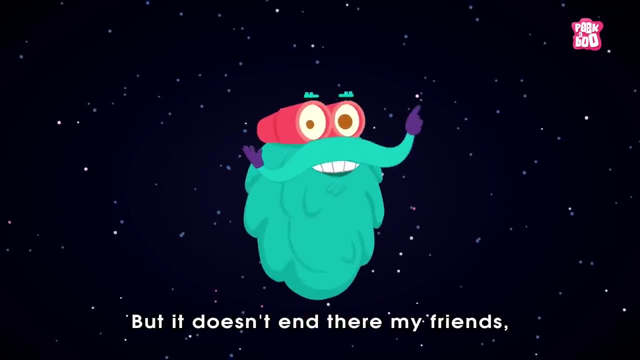 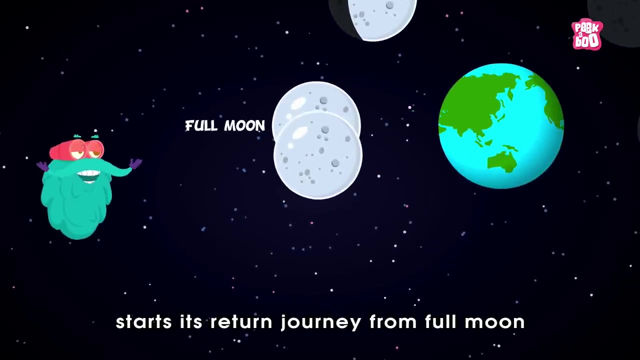 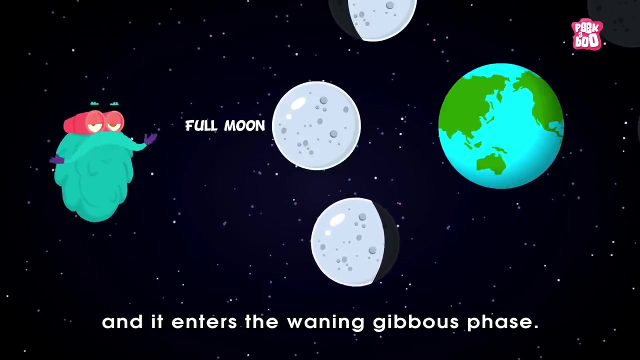 due to which, finally, we can see the Full Moon, But it doesn't end there, my friends, as now comes the Waning Stage, where the Moon starts its return journey from Full Moon to the Invisible New Moon, as the light begins to decrease on its surface. 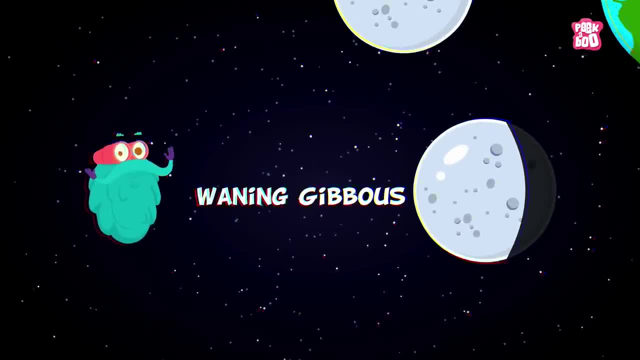 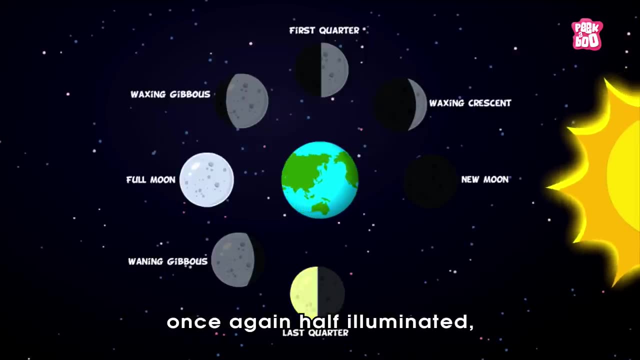 and it enters the Waning Gibbous Phase. After this occurs, the Last Quarter Phase, during which the Moon is once again half-illuminated, but the lit area that's visible is on the decline. This is followed by the Waning Crescent Phase. 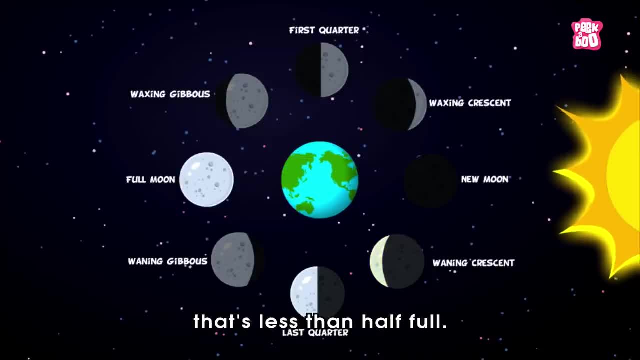 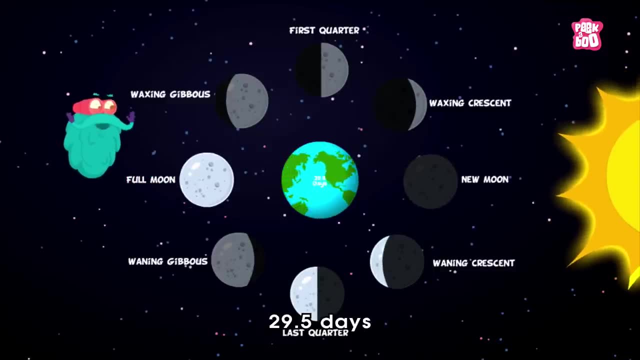 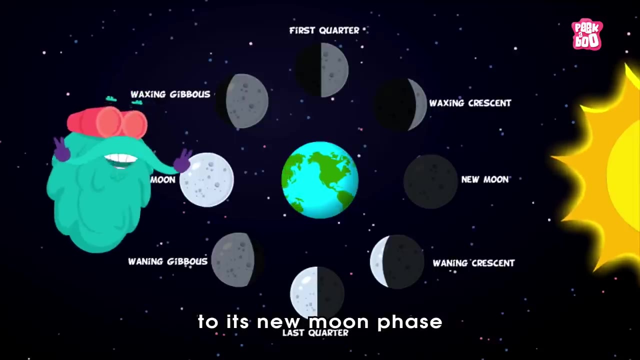 in which the Moon shrinks back to a crescent that's less than half full. And finally, the Moon finishes its journey in about 29.5 days and comes back between the Earth and Sun to its New Moon Phase, marking the completion of the Lunar Cycle. 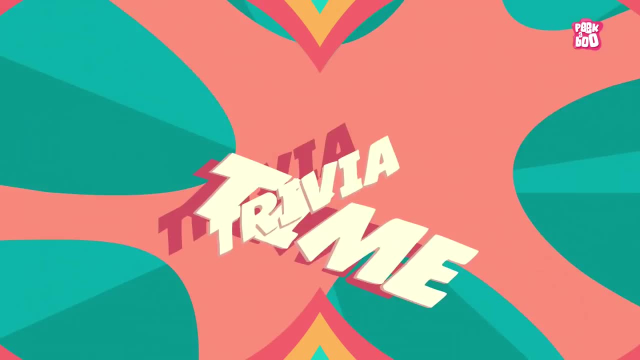 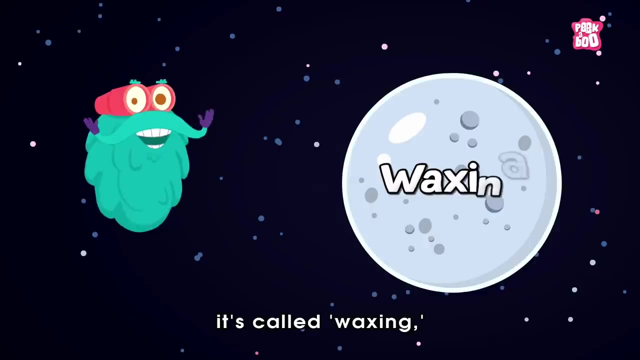 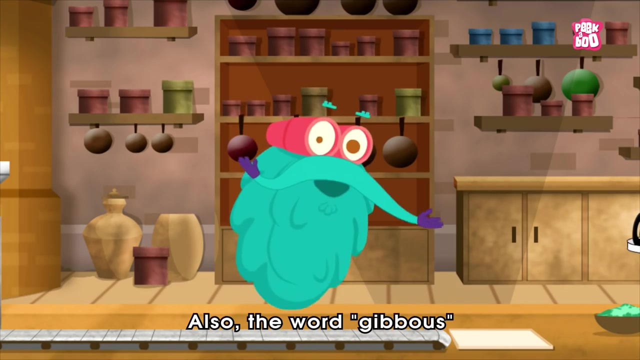 just to start over again TRIVIA TIME. Did you know? when the Moon appears to be getting bigger, it's called Waxing, and when it looks like it's getting smaller, it's called Waning. Also, the word Gibbous comes from the Latin for Hump.